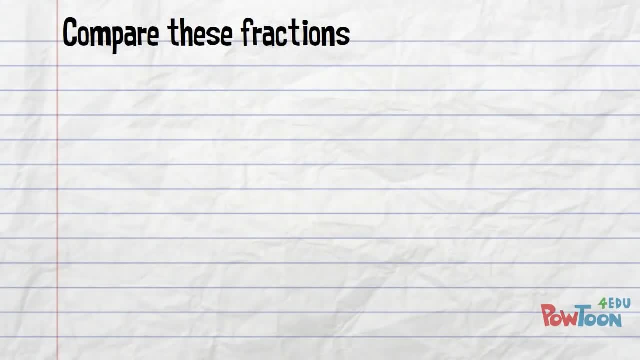 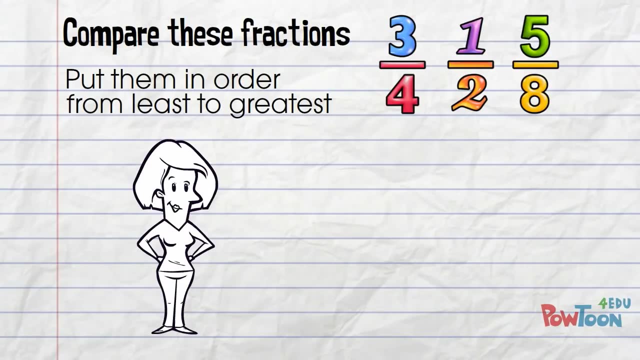 Let's say we have to compare THESE fractions, We have to put them in order from LEAST to GREATEST. We think our way through the problem. One strategy is to use fraction strips And remember fraction strips are all the same length. 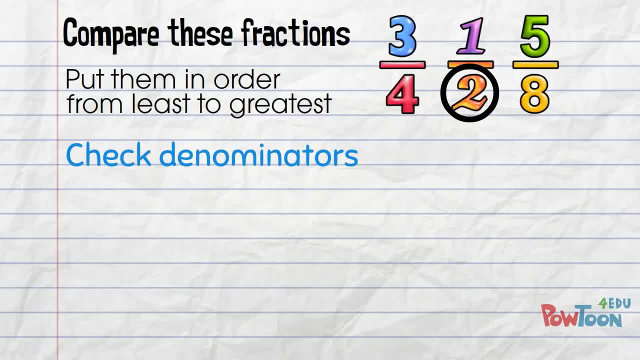 First we check. the denominators 2 and 4 are BOTH factors of 8. So all the fraction strips can be 8cm long. I do the fraction with the LARGEST denominator first. Always use a ruler to make your fraction strips. 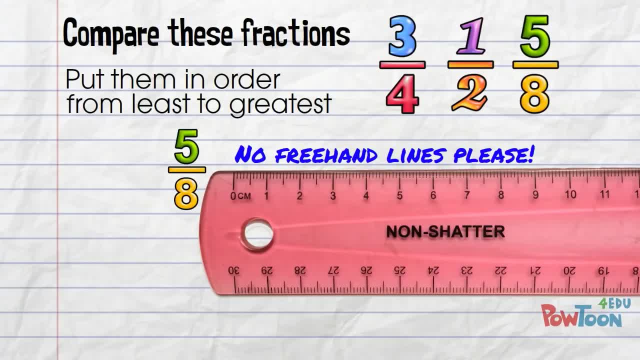 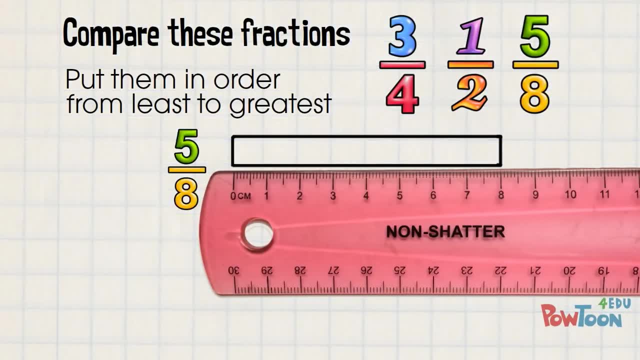 No free hand lines please. It's math, not art. 1 fraction strip 8cm long, or 8 squares long if you happen to have squared paper in your math book. Each centimeter is 1 part out of 8.. Now I colour in the fraction value: 5 eighths. 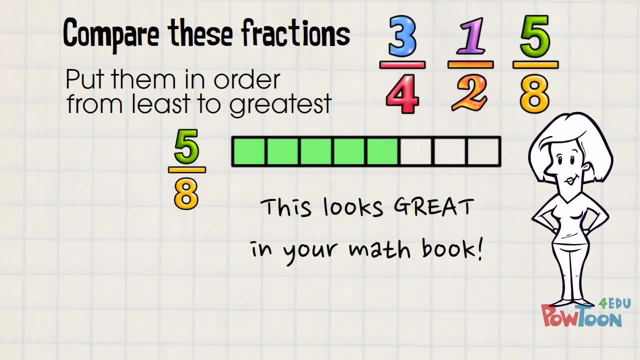 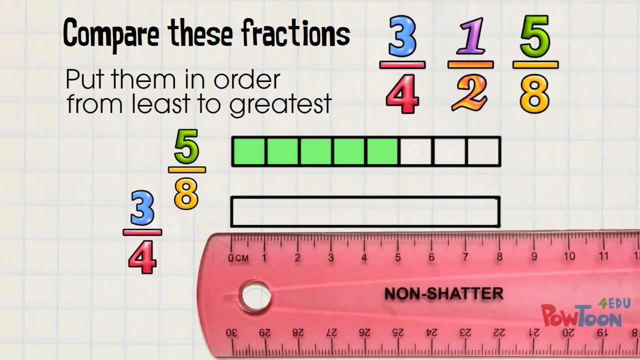 If you colour in your fraction strips carefully, it looks great in your math book. Next I go to 3 quarters. We know the fraction strips all have to be the same size, so I make another section. I do the fraction strip 8cm long, in line with the last strip. 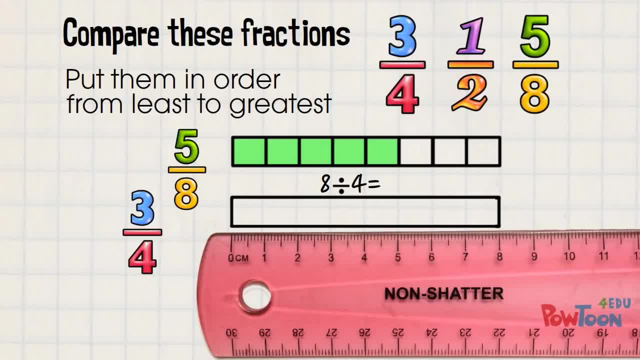 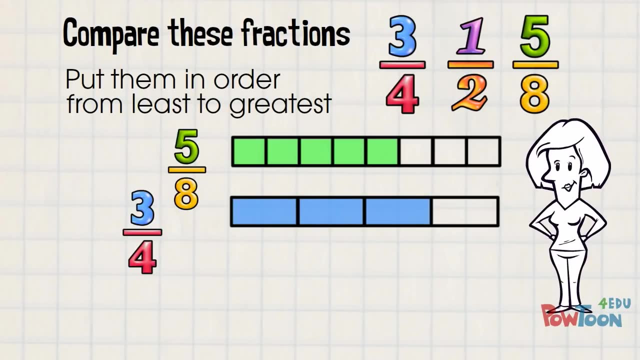 The denominator is 4, so I say 8 divided by 4.. That gives me 2cm for each part, 4 parts. each part is 1 quarter. Then I colour in 3 quarters on the fraction strip. Last I do the fraction with the smallest denominator, the half. 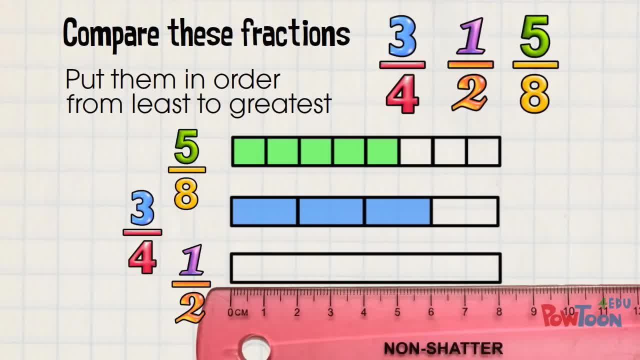 8cm divided in 2 tells me each half is 1.5cm. 8cm divided in 2 tells me each half is 1.5cm. 7cm divided in 2 tells me each half is 4cm. 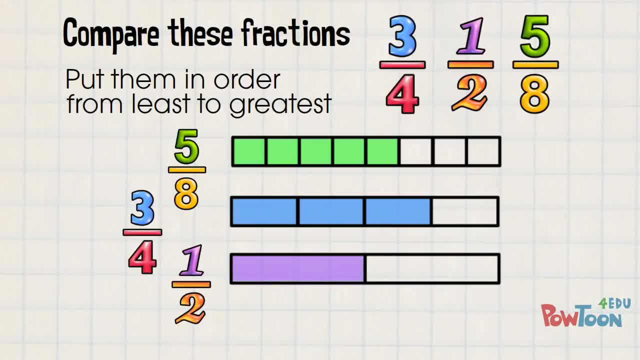 8cm divided in 2 tells me each half is 2.5cm. 7cm divided in 2 tells me each half is 4cm. And I colour my half. Because these fraction strips are lined up vertically, we can see easily which is biggest and smallest. 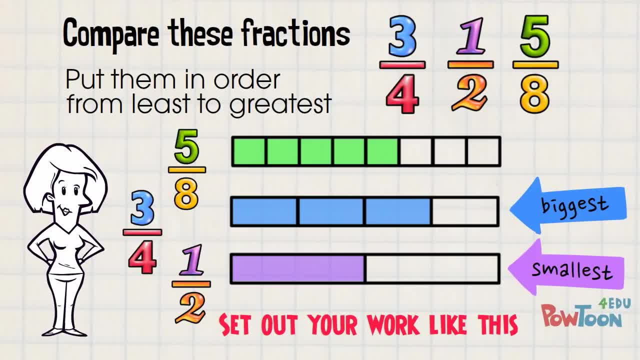 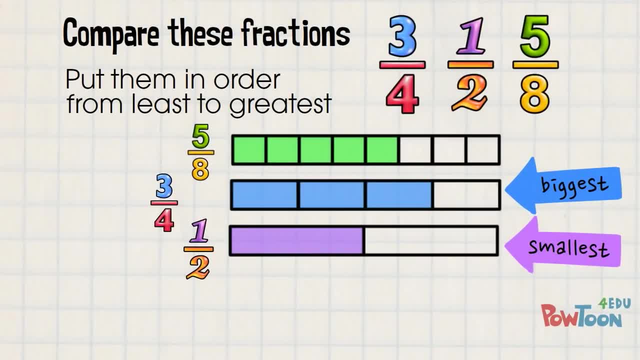 I'd like you to set out your work like this too. Then we simply write a math statement of what we found using the appropriate math sign. The problem set put the fractions in order from least to greatest. So don't get it wrong now.